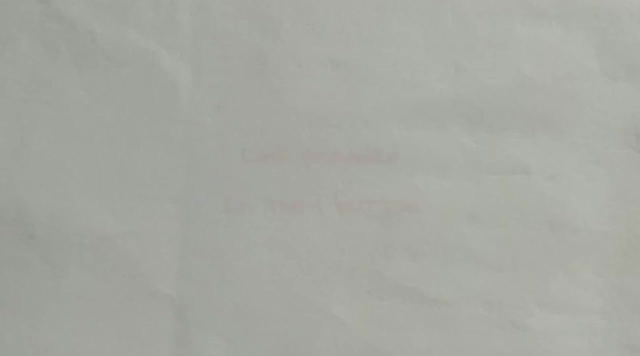 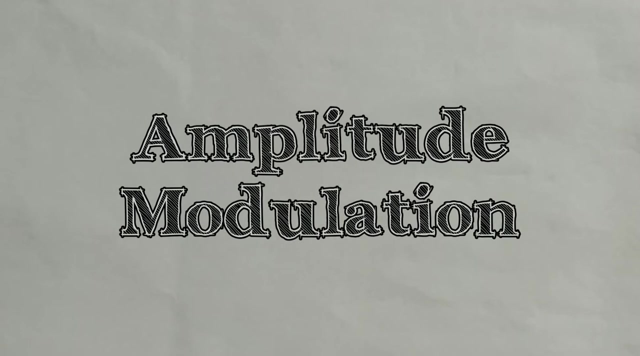 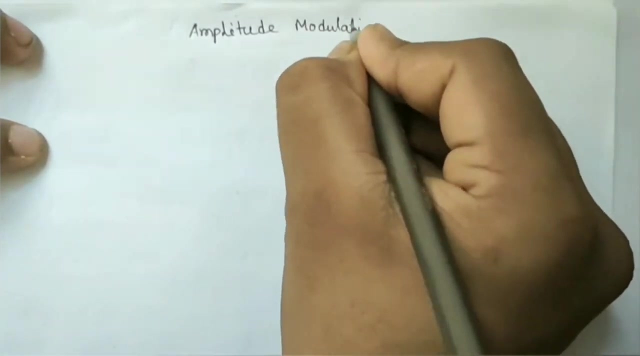 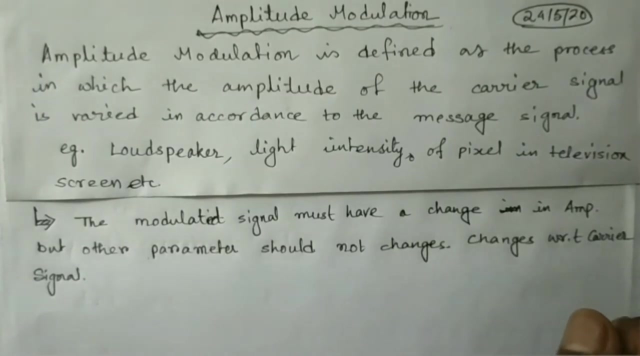 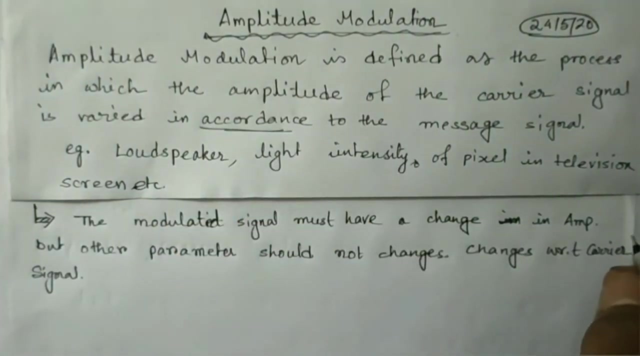 Welcome. In the last video we had discussed about the basics of communication and communication system. Today we will discuss about the amplitude modulation. As said earlier, amplitude modulation is defined as the process in which the amplitude of the carrier signal is varied in accordance to the message signal. The modulated signal must 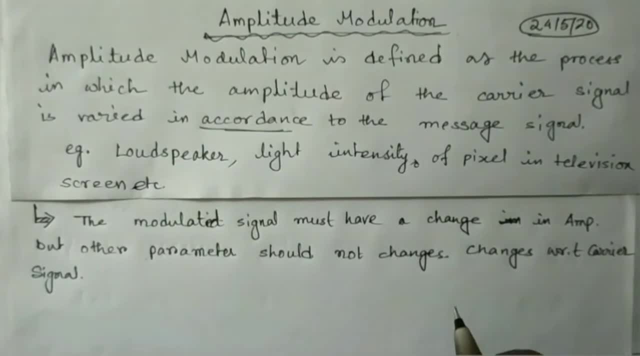 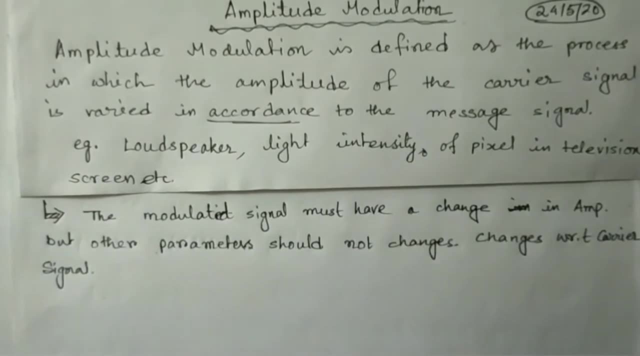 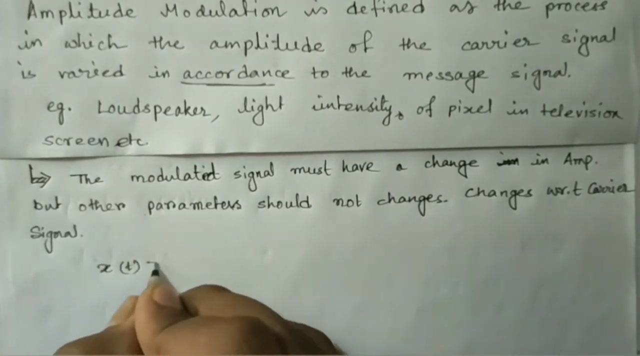 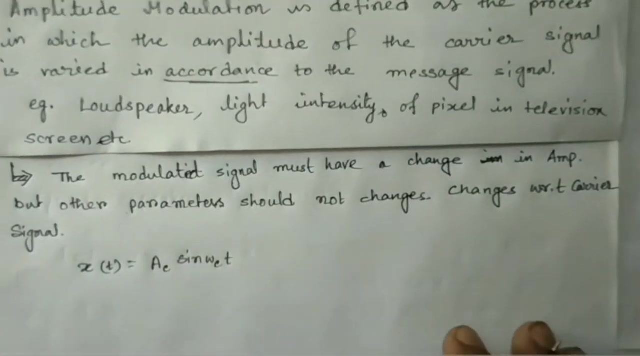 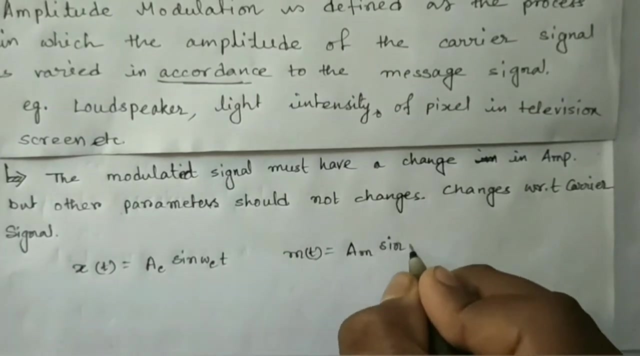 have a change in amplitude, but the other parameters, like phase or frequency, should not change And changes are with respect to the carrier signal. Suppose the carrier signal is Xt equals to Ac And the message signal is mt equals to Am, sin, omega, mt. And if you represent them graphically, 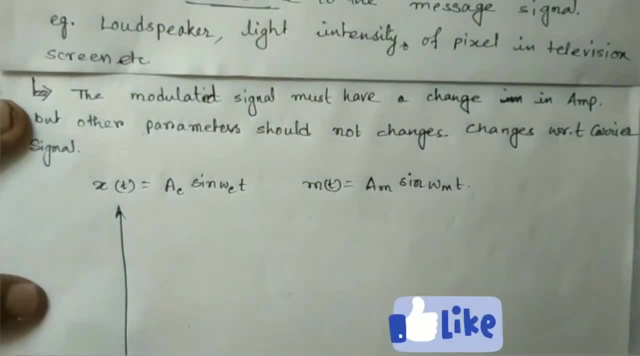 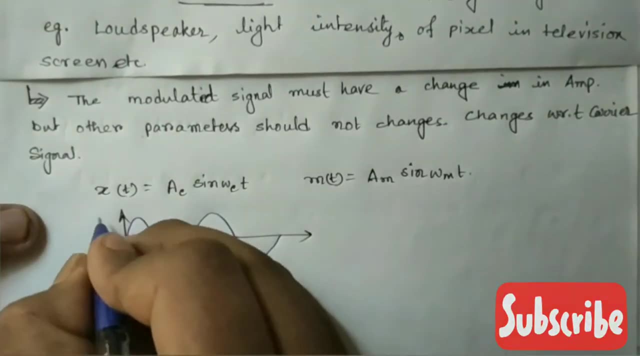 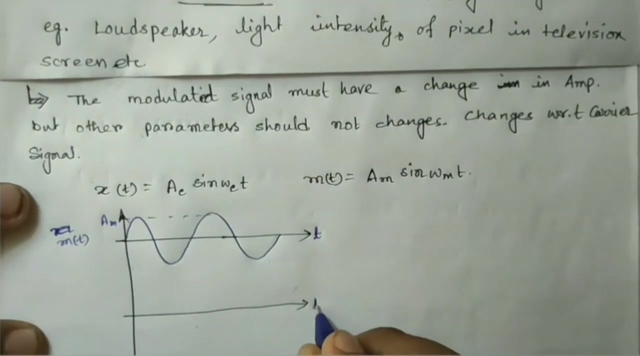 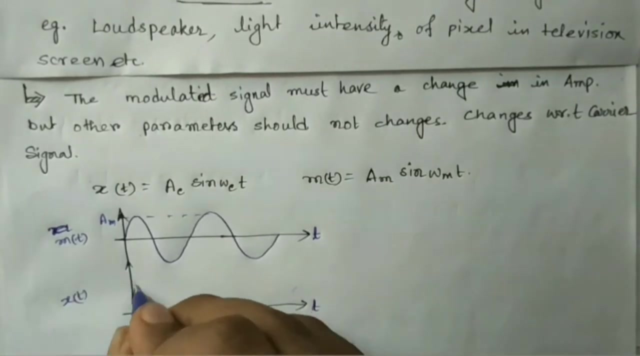 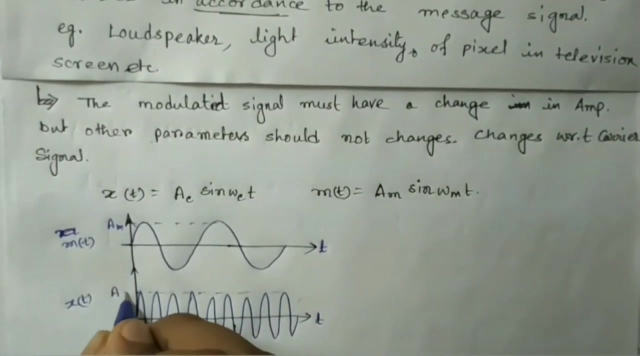 then this is the message signal, mt, and the amplitude is Am. The frequency of the carrier signal is higher than the frequency of the message signal. So the Xt will be like this And the amplitude is Ac, And the modulated signal will be this: 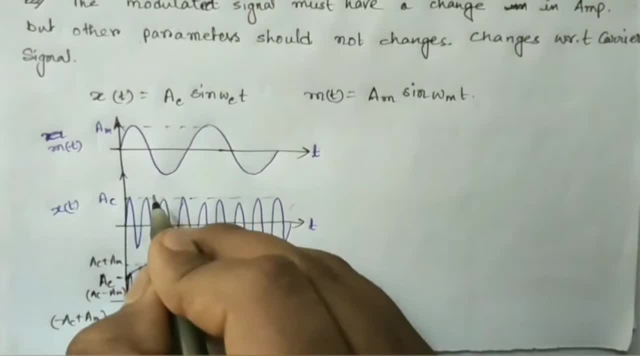 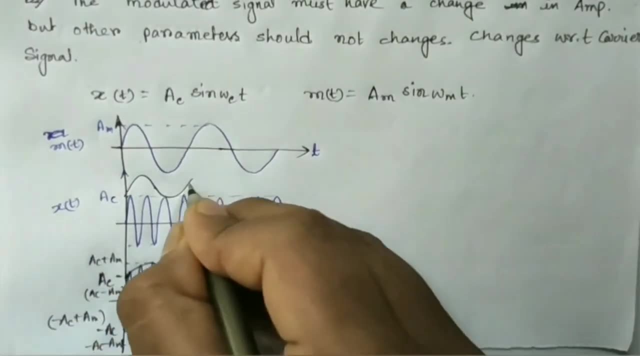 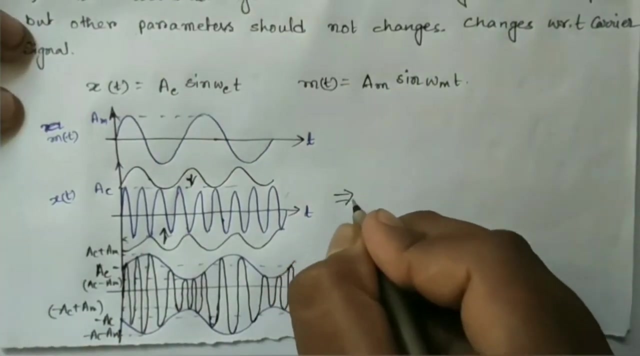 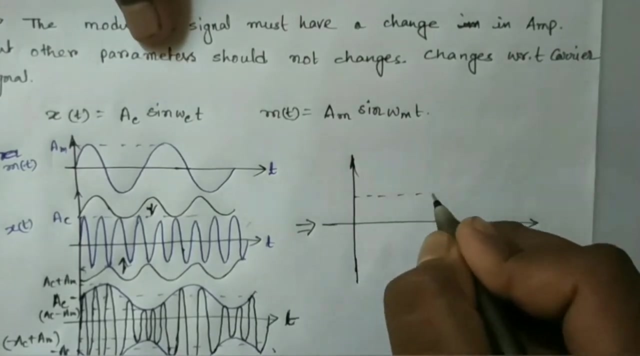 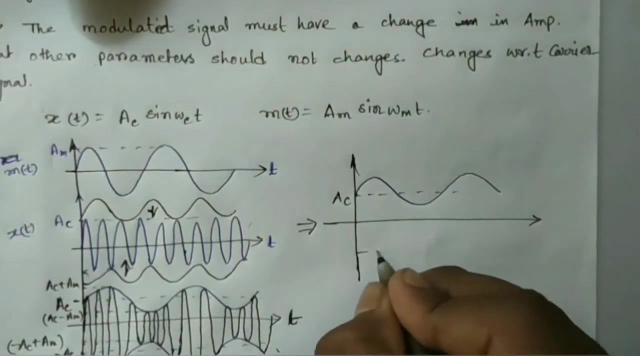 The amplitude modulated signal is attained by adding the message signals from both directions, in positive and negative directions. They are added like this: Suppose this is Ac When this message signal is added to it, then the output signal will be like this: And on the negative side, also: suppose this is minus Ac When this signal 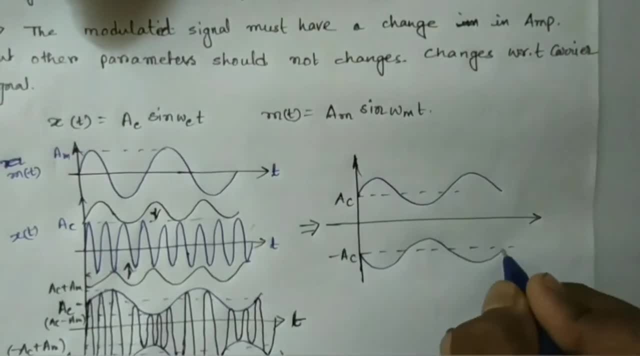 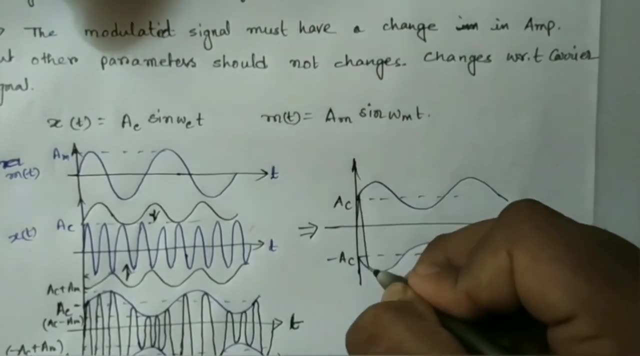 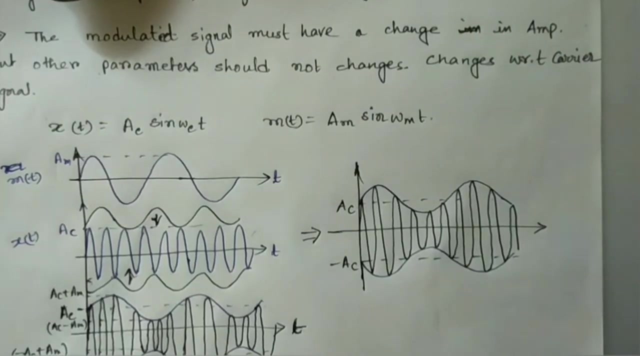 is added, then the output signal will be like this, And thus we attain the modulated signal Here. this is the message signal with frequency Omega-m, Whereas this is the carrier with frequency Omega. that is how the modulated signal is attained. 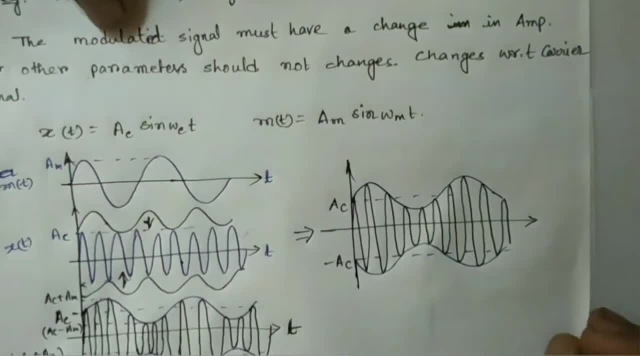 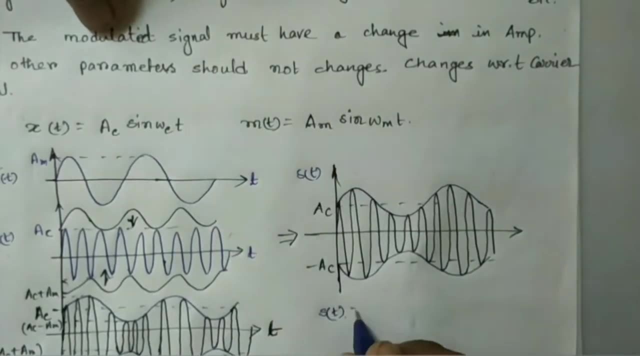 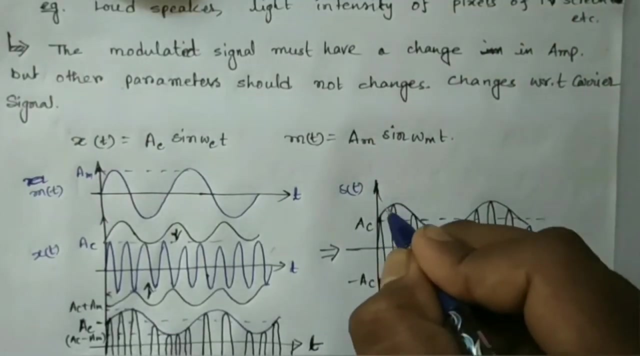 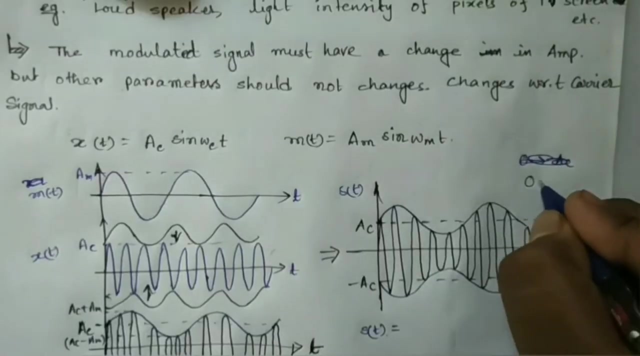 Now from this we can get the equation of modulated signal which is given by S of t. In the modulated signal there will be a change in amplitude Here about this Ac. the output is varying, like the message signal. this signal was initially at zero origin. when origin is: 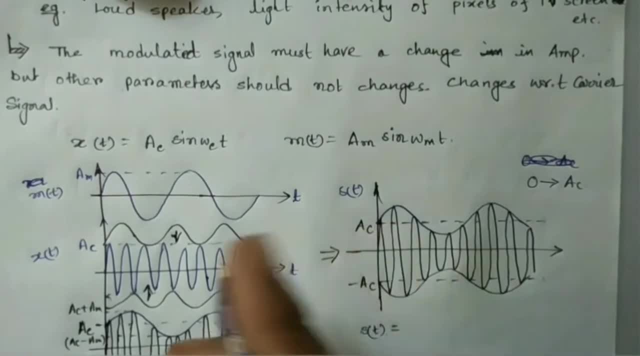 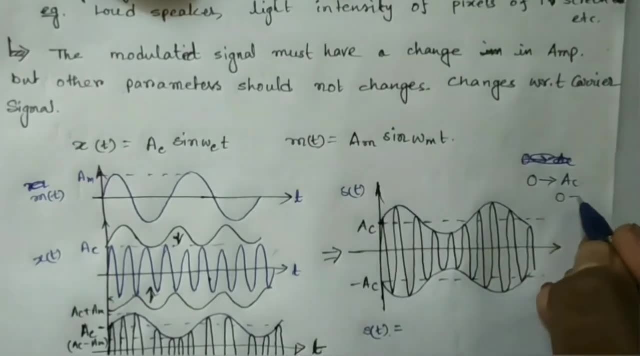 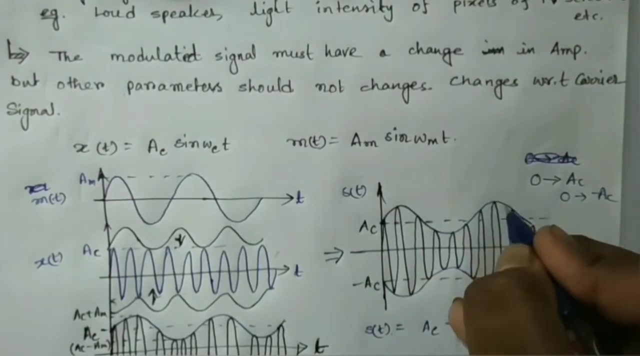 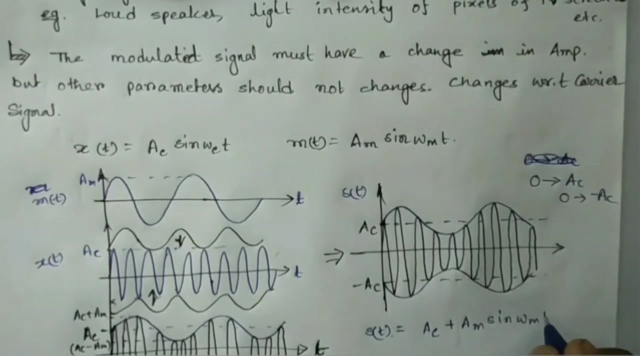 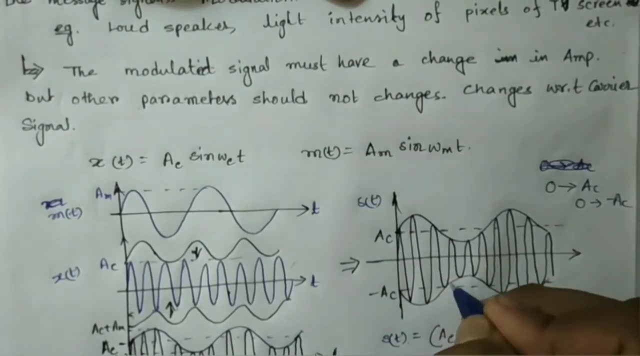 shifted from zero to ac, this signal is shifted to ac, so the output will be like this: and when the origin is shifted to minus ac, then this will be the output. so st is equals to ac plus. this variation is mt, or am sine omega mt, and this frequency is frequency of carrier. 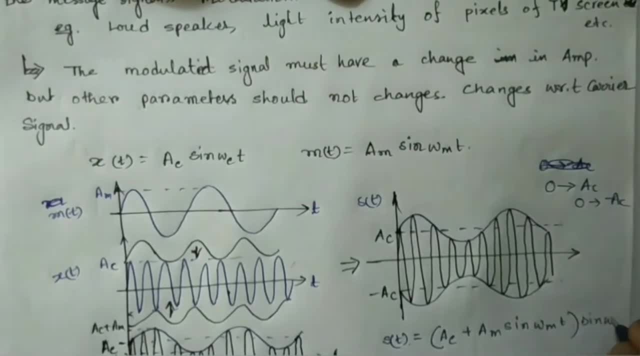 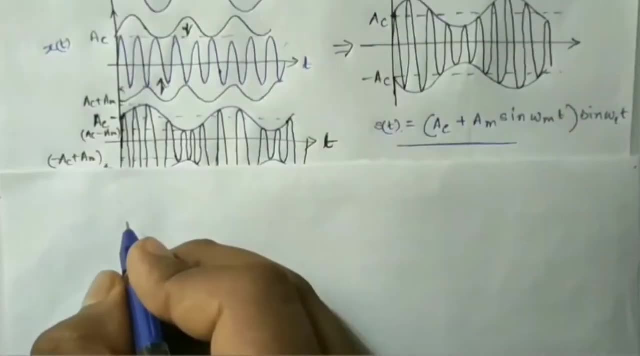 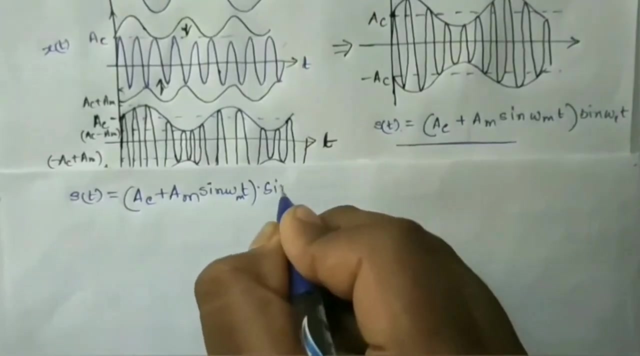 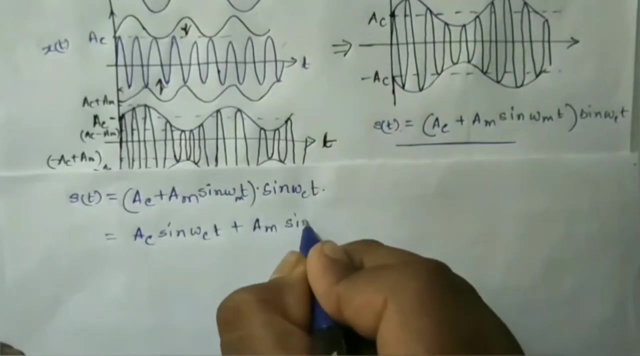 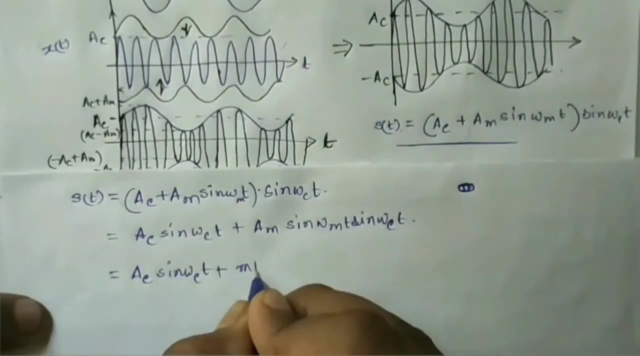 signal, so sine omega ct. so this is the equation for the modulated signal. so we have AC equals to AC plus AM sine omega mt into sine omega Ct. so let us solve this: AC sine omega Ct plus AM sine omega mt into sine omega Ct, that is, AC sine omega Ct plus M. AC into half, into two, sine omega mt into sine. 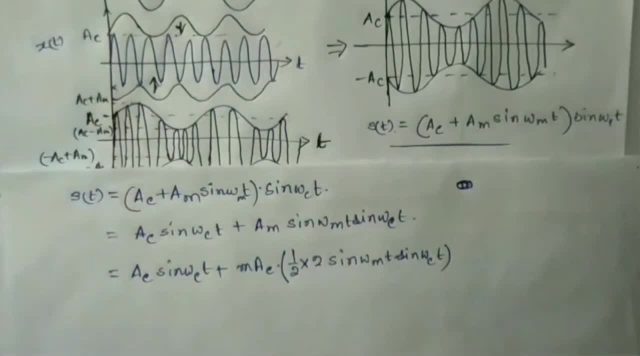 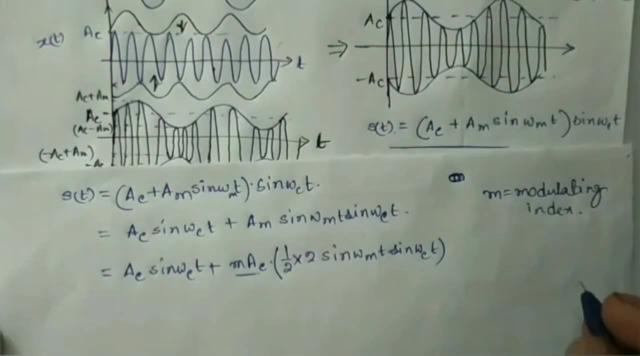 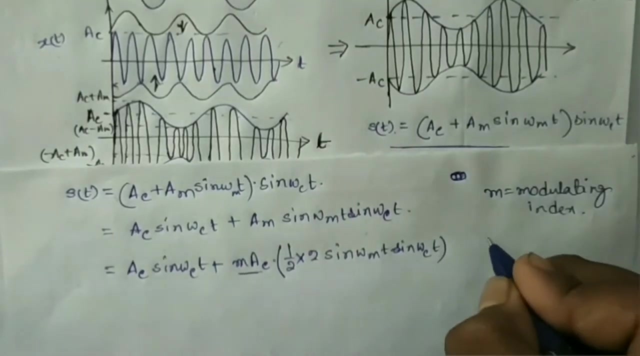 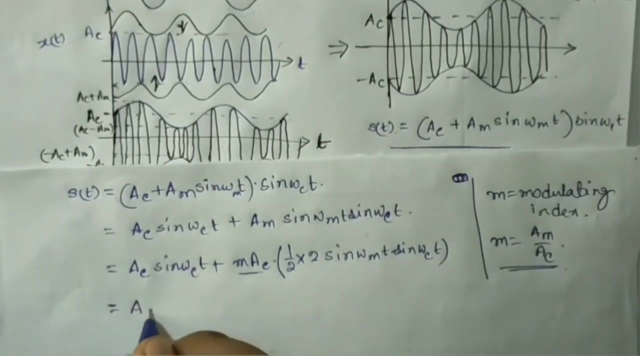 omega Ct. here this EM is replaced by MAC, while M is the modulation index for tällation and it is defined as the ratio of amplitudes of M, 머�r signal and carrier signal. so M is AM by AC, that is, AM is equal to M, AC, so AC into sine. 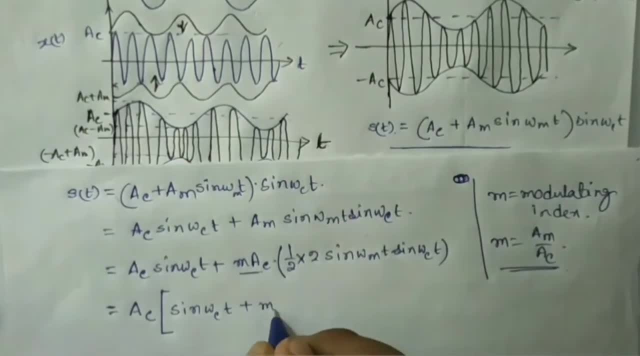 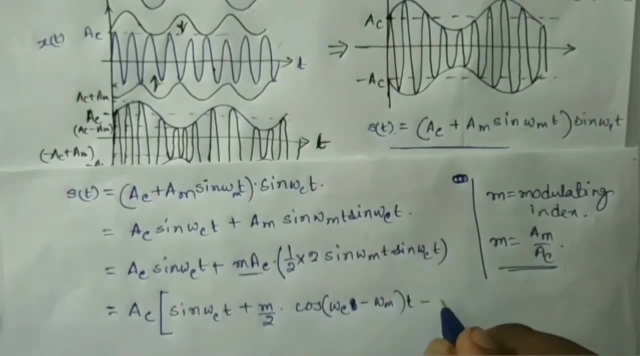 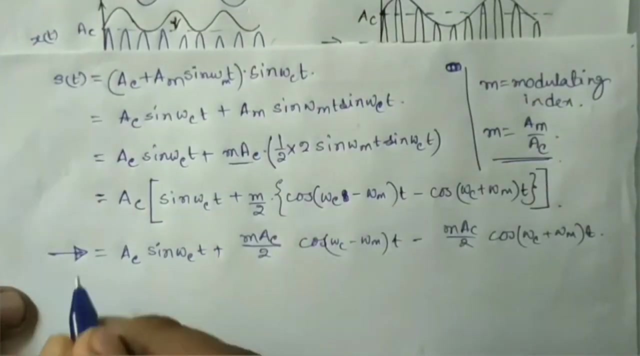 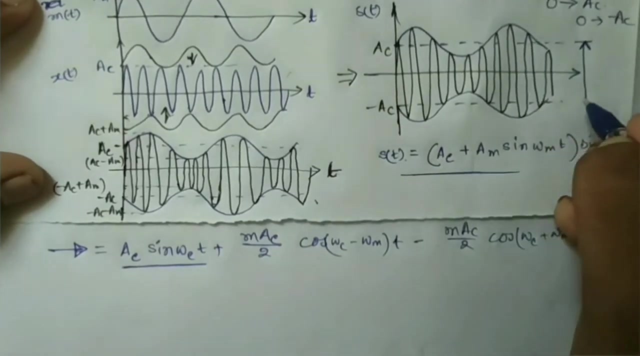 omega Ct plus tick 2 into cos of omega c minus omega m into t, minus cos of omega c plus omega m into t. so this is the equation for the modulated signal. here this ac sine omega c, t turn is the signal for this region, m ac by 2. cos omega c minus omega mt is the lower sideband. 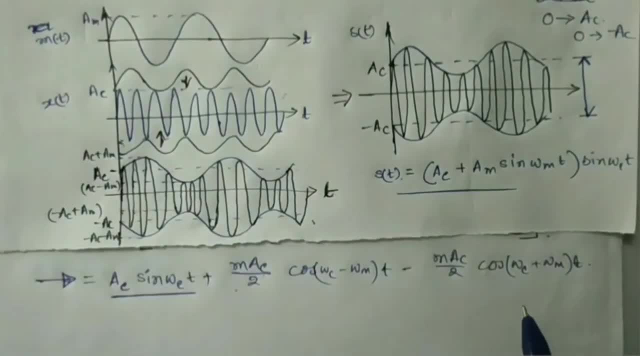 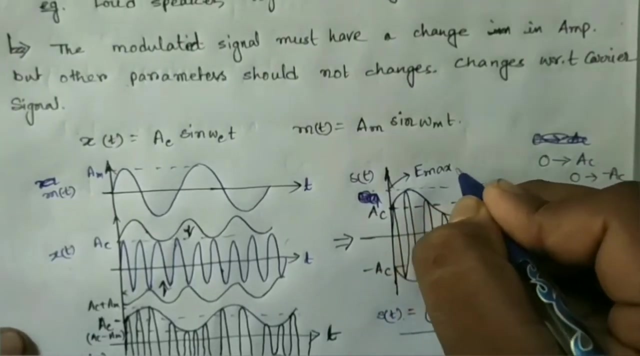 and m ac by 2 cos. omega c plus omega mt is for the upper sideband. the bandwidth required to transmit these signals is 2 omega m and the operating frequency is this carrier signal frequency: omega c, suppose this is e max and this is e min. 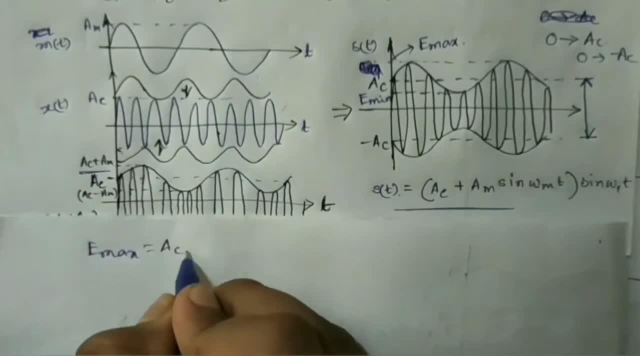 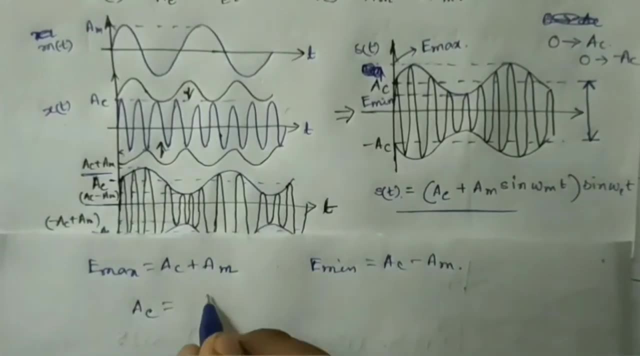 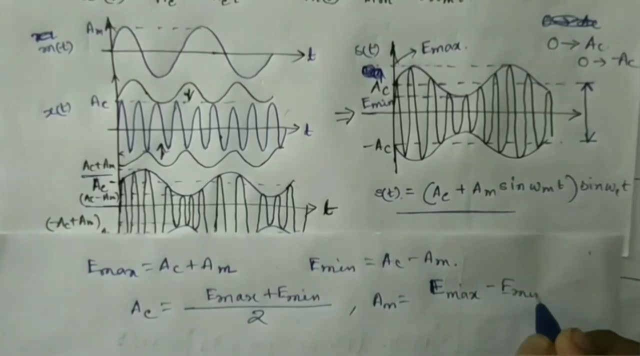 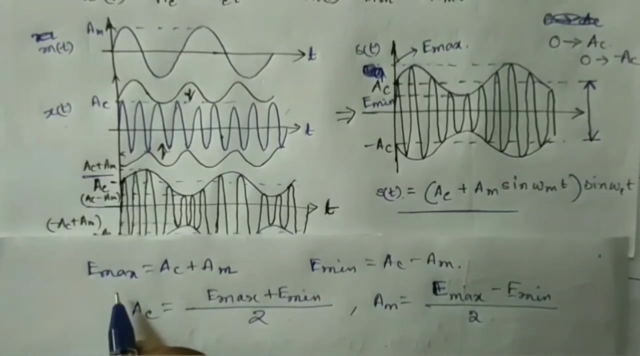 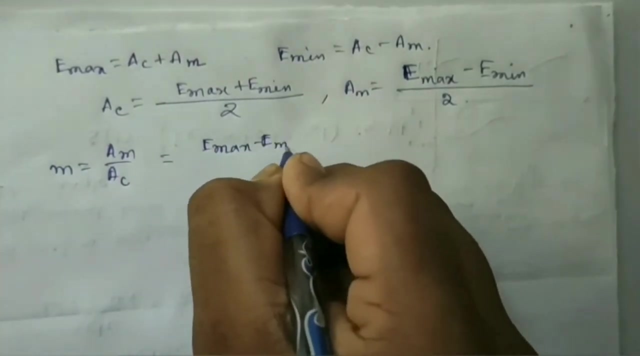 so. So emax is ac plus am and emin is ac minus am. that is, ac is emax plus emin divided by 2 and am is emax minus emin divided by 2.. And modulation index m being am by ac, it will be emax minus emin divided by emax plus emin. 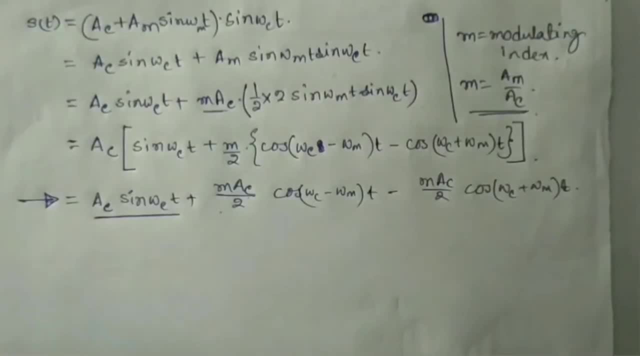 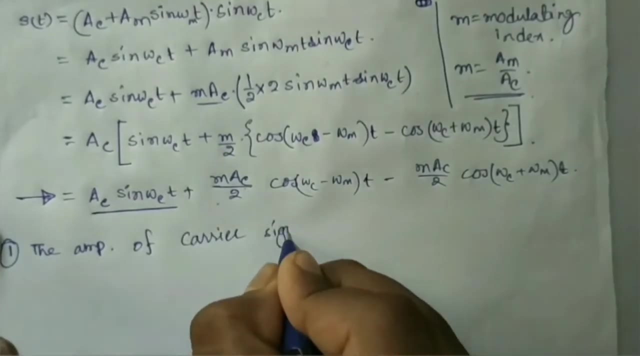 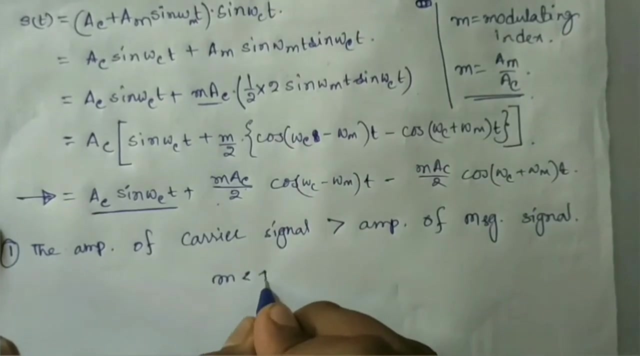 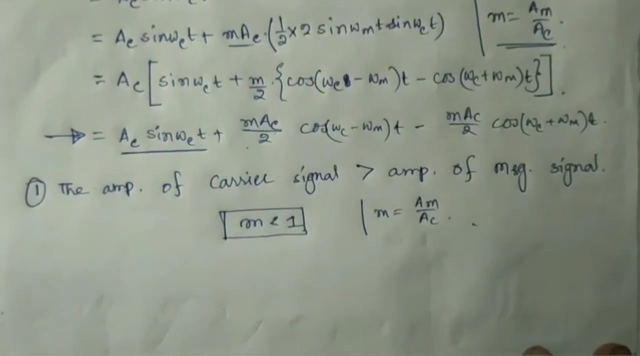 this is very important for numericals. Now let us see some important points. First is amplitude of the carrier signal must be greater than the amplitude of message signal, And since am is am by ac, m will be less than 1.. Okay, Now let us justify this point. 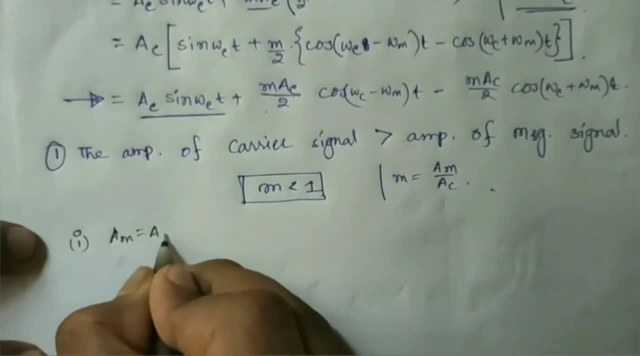 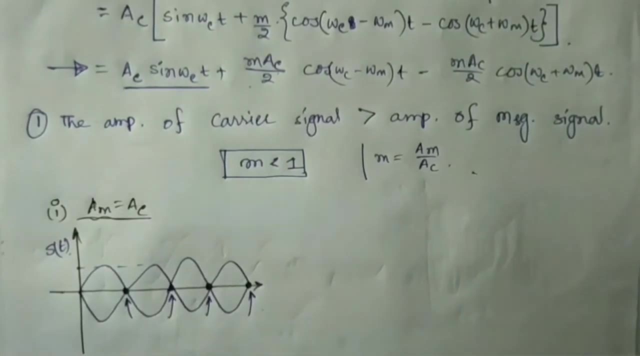 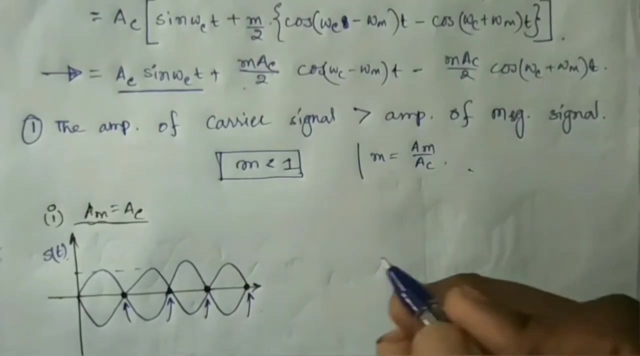 Suppose m is equals to ac. For this case, this is our output graph. At this nodes we are getting zero voltage. hence we cannot make out that, whether it is a fault of the machine or actually, the input is zero. So this is not desired. 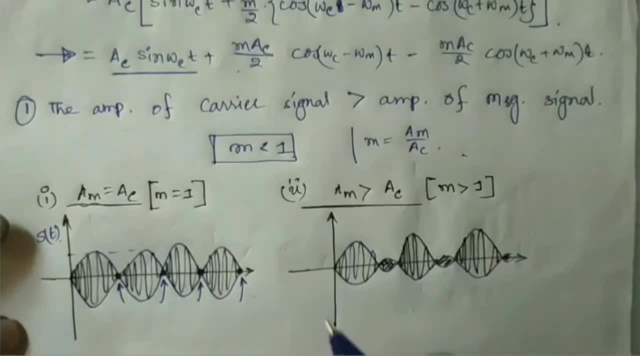 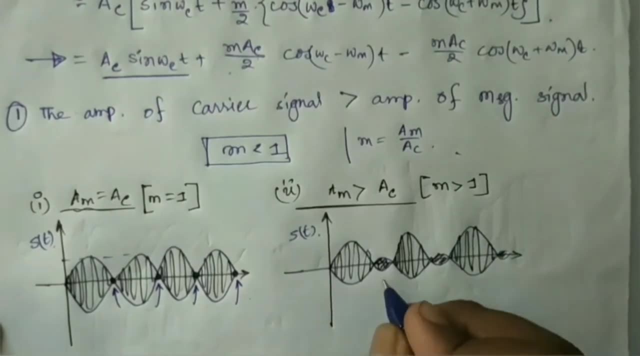 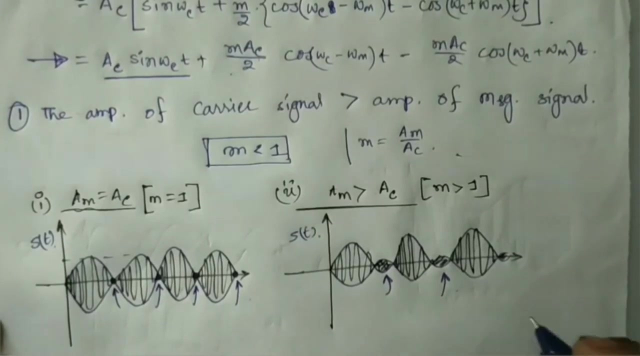 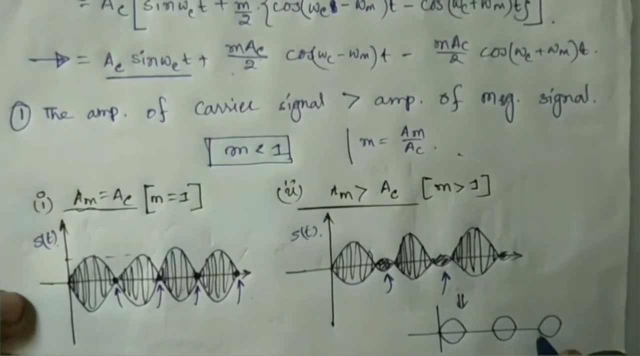 Hence am should not be equals to ac. For am greater than ac, that is, for m greater than 1, the output graph will look like this Here: at these points the carrier signal is overlapped and they are getting cancelled, So the output of this is a discrete value. 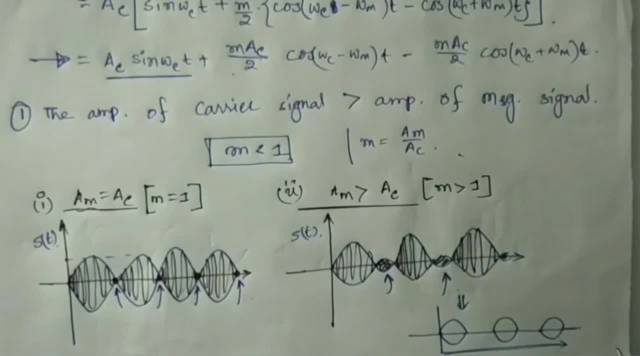 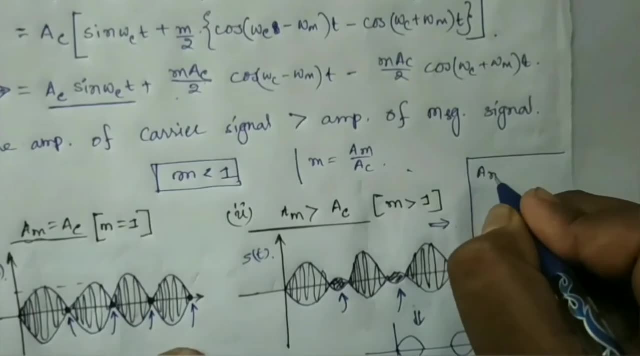 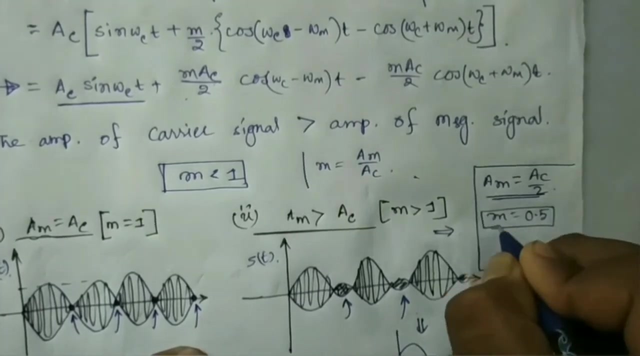 And when we will demodulate this signal. we cannot get the actual message signal. So this condition is also not desired. The best case is When am is ac by 2, that is, am is 0.5. For this condition we will get a pure and perfect modulated signal which can be demodulated. 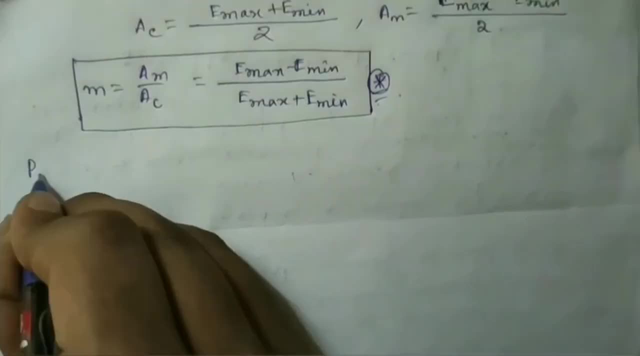 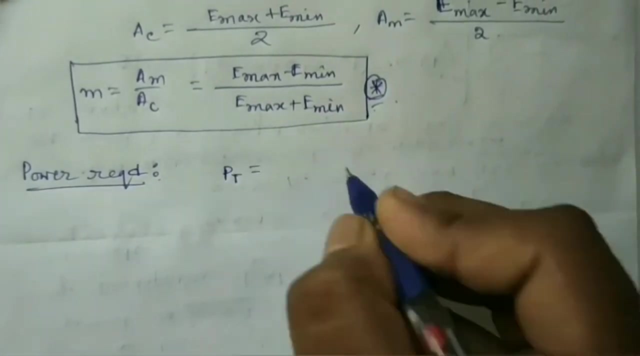 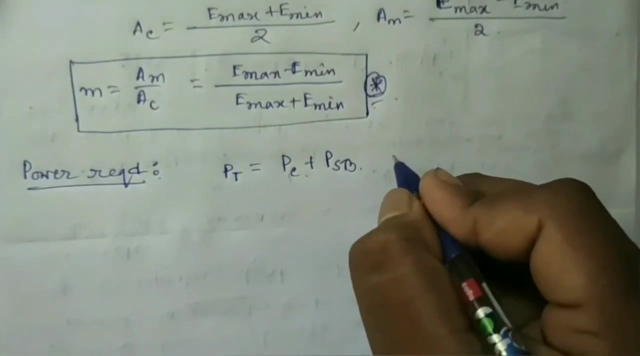 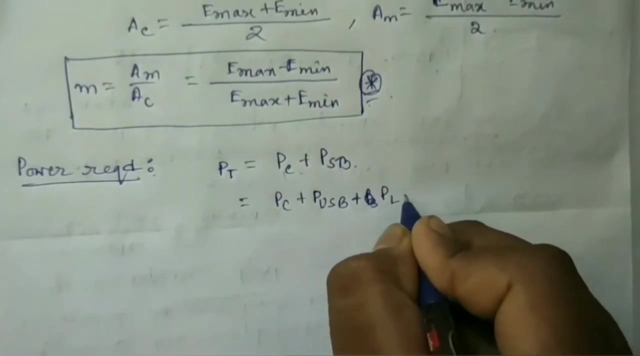 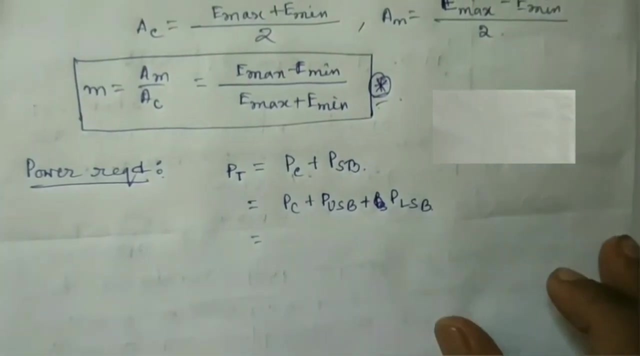 very easily. Now, total power required to transmit the signal is pc plus psb, that is a power to transmit carrier signal and the sidebands. So it is equals to pc plus pusb plus plsb. Now here, power p is v into i, that is v square by r, and all analog signals are in the form. 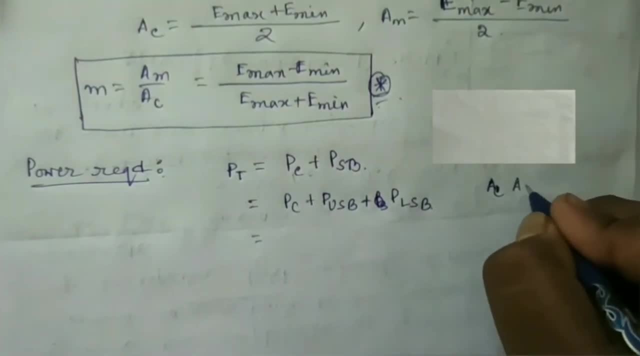 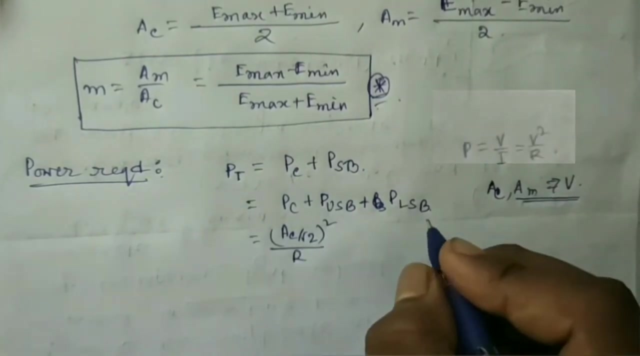 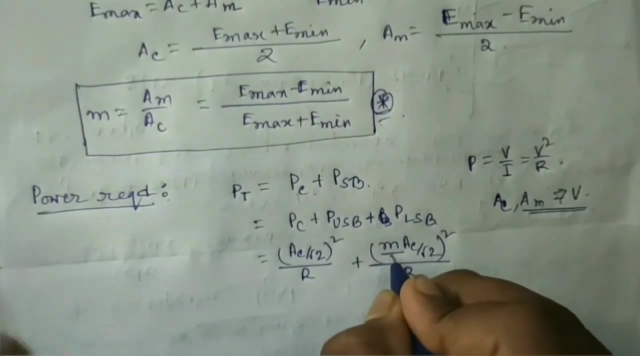 of voltages, So ac, am. these are all representing voltage. Here we will use the rms value. So pc will be ac by root: 2 whole square divided by r. p, usb will be m, ac by root, 2 whole square divided by r, and half will be multiplied because. 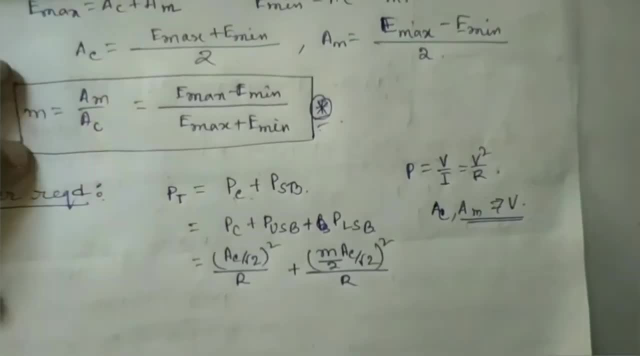 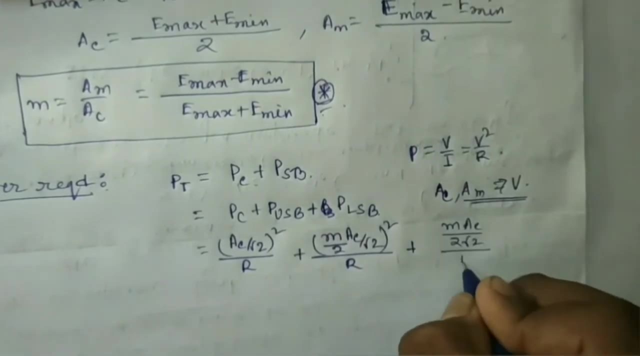 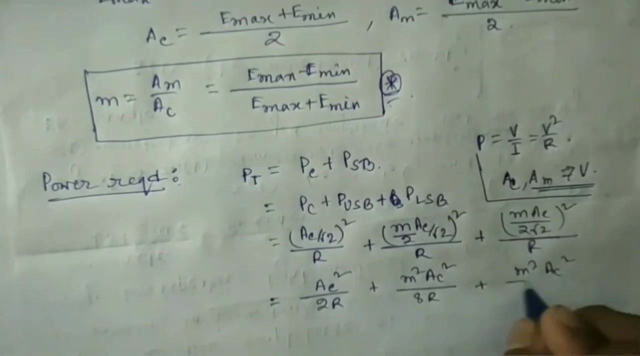 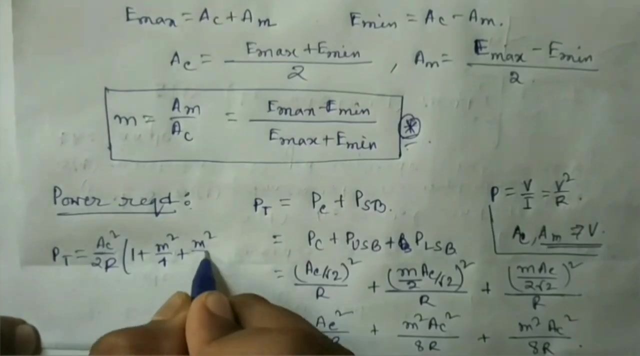 of this And similarly p lsb will be m ac by 2 root 2 whole square by r. That is equals to ac square by 2 r plus m square ac square by 8 r. So pt is ac square by 2 r into 1 plus m square by 4 plus m square by 4.. 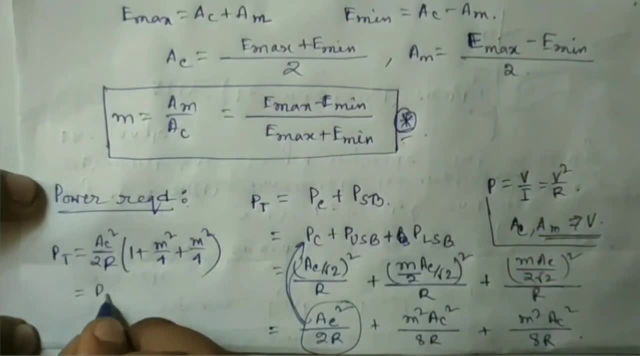 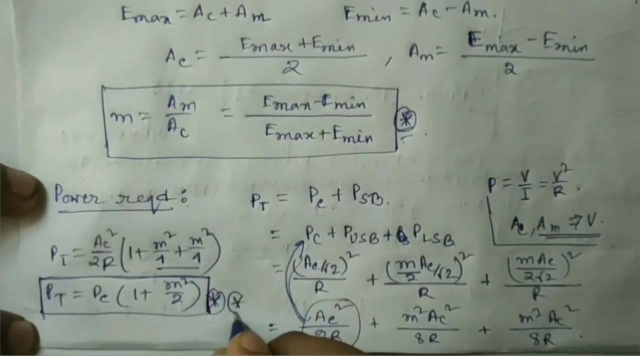 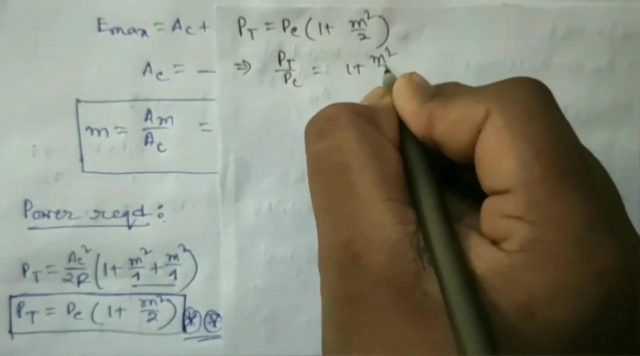 Here ac square by 2. r is the pc, so pc into 1 plus m square by 2.. This equals to pc and it is very important for numericals. Now, from here, pt upon pc will be 1 plus m square by 2.. 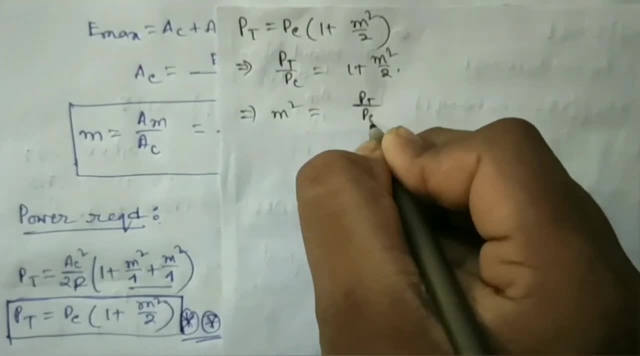 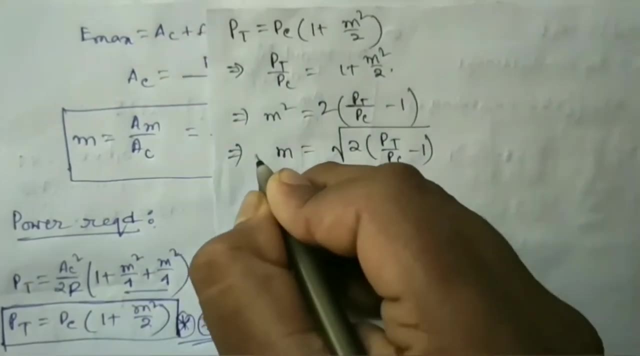 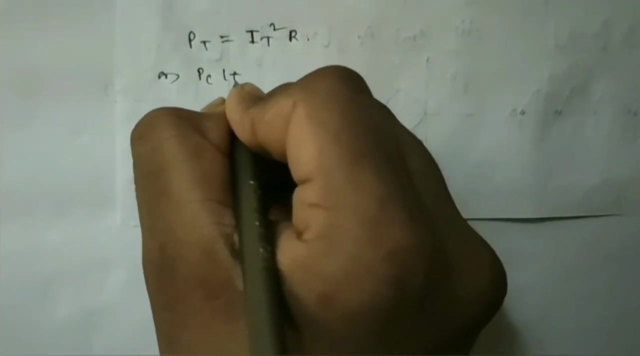 That is m square is pt by pc minus 1 into 2 and m will be root over of 2 into pt upon pc minus 1.. Again, we know: pt is it square into r, pt is pc into 1 plus m square by 2.. 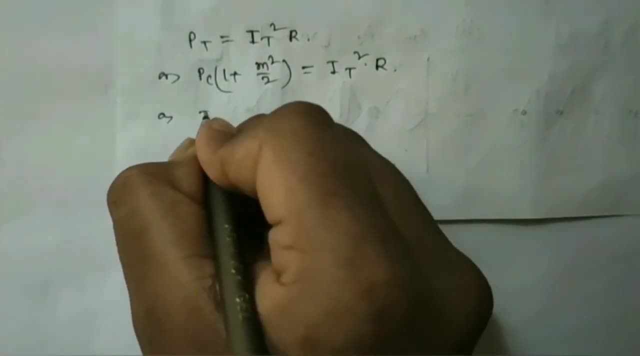 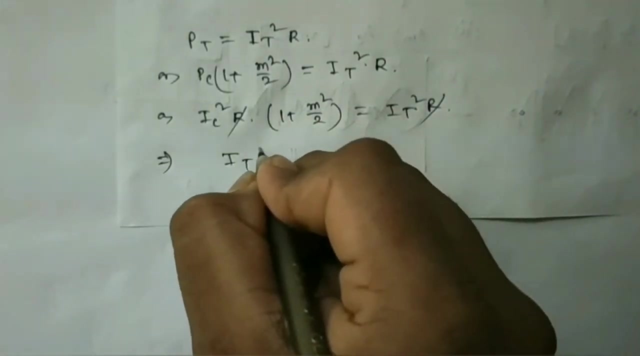 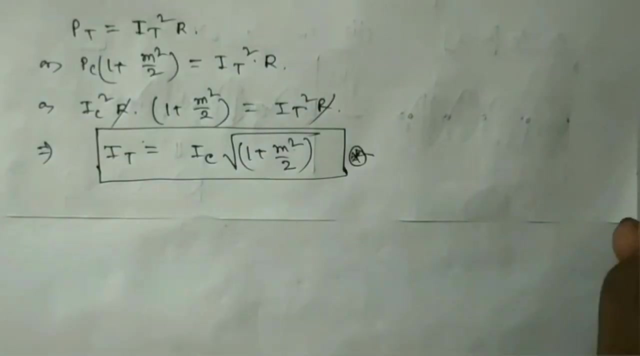 That is equals to it square into r. Now, pc is ic square into r, So from here we will get It square equals to ic square into 1 plus m square by 2.. That is, it is ic into root over of 1 plus m square by 2.. 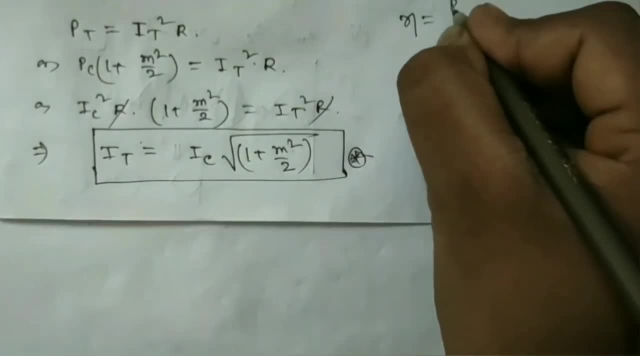 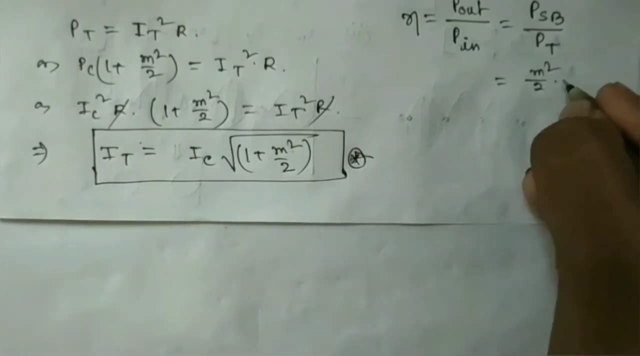 Now let us calculate the efficiency. So eta is p out by p in. p out is the power to transmit the sidebands and p in is total power. psb will be m square by 2 into pc and pt is pc into 1 plus m square by 2.. 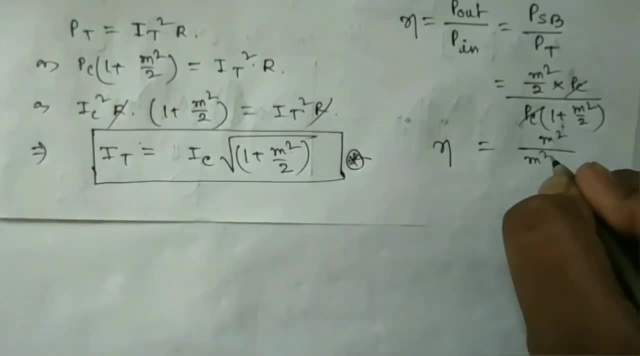 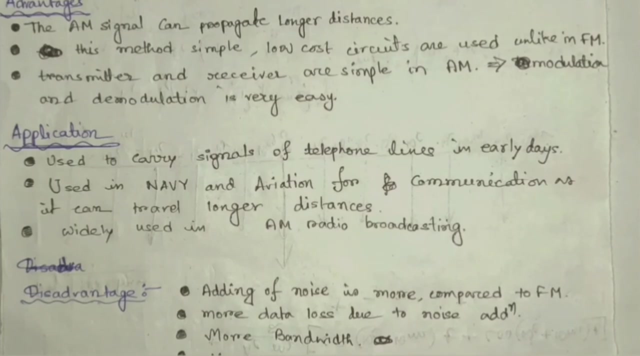 That is, eta will be m square by m square plus 2.. And in percentage, eta's value will be m square by m square plus 2 into 100 percent. This is very important for numericals. Now let us see what are the advantages of amplitude modulation. 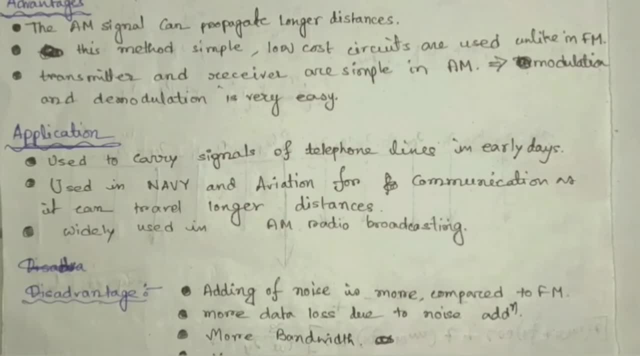 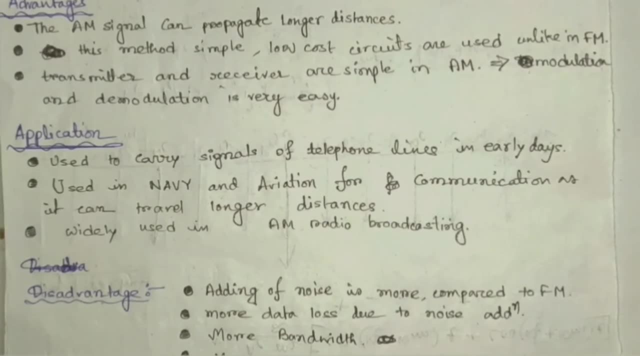 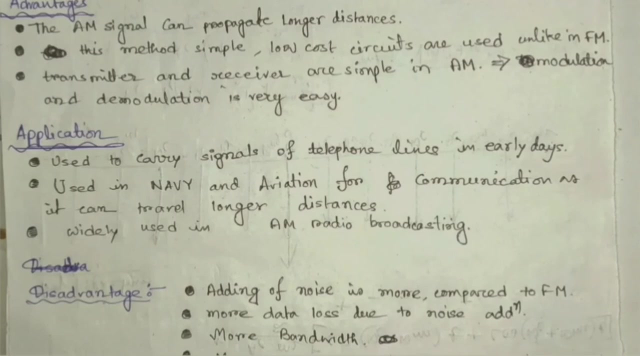 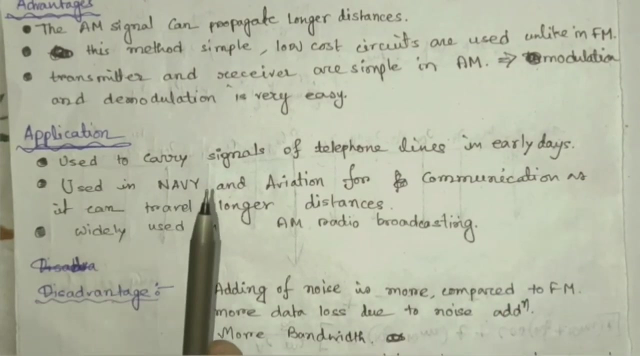 Amplitude modulated signal can propagate longer distances as the amplitude is modified. This method is very simple and low cost circuits are used, unlike in frequency modulation, And transmitters and receivers are very simple in amplitude modulation circuit And hence modulation and demodulation is very easy. 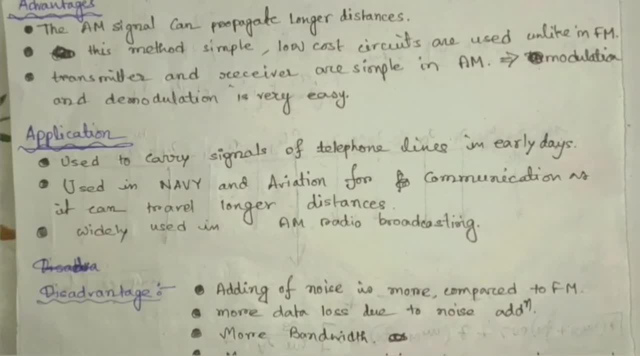 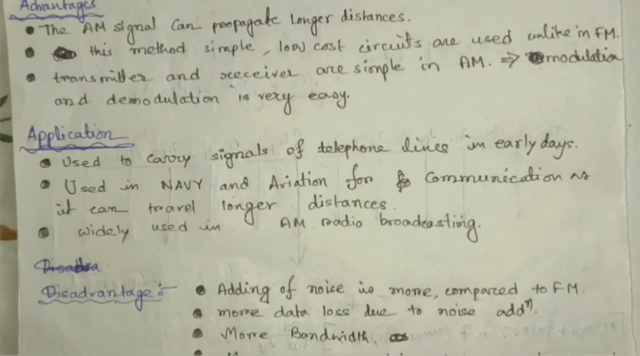 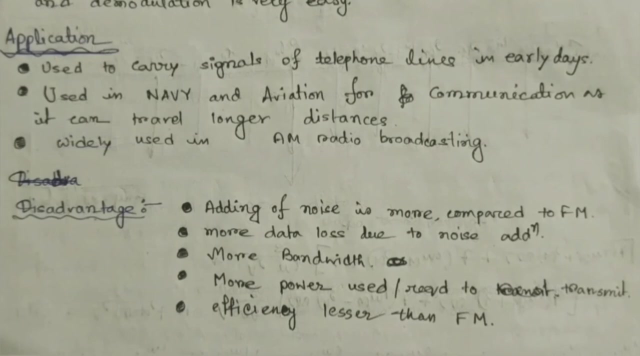 Amplitude modulation was used to carry signals of telephone lines in early days. It is used in navy and aviation for communication as it can travel longer distances, And it is widely used in am radio broadcasting. But amplitude modulation has several disadvantages. also, Addition of noise is higher in amplitude modulation than in frequency modulation. 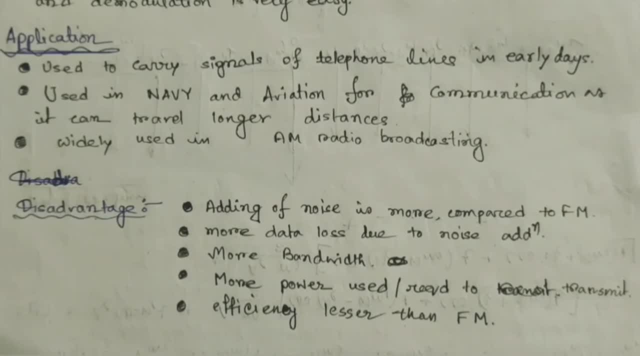 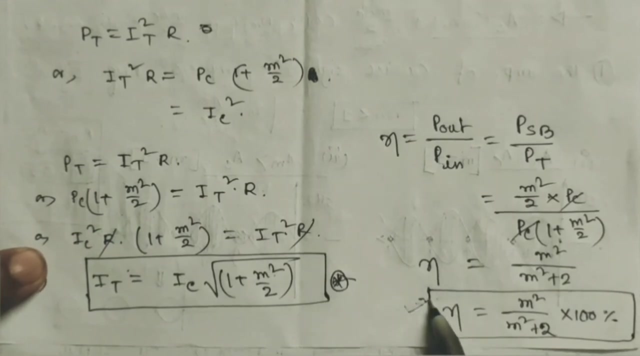 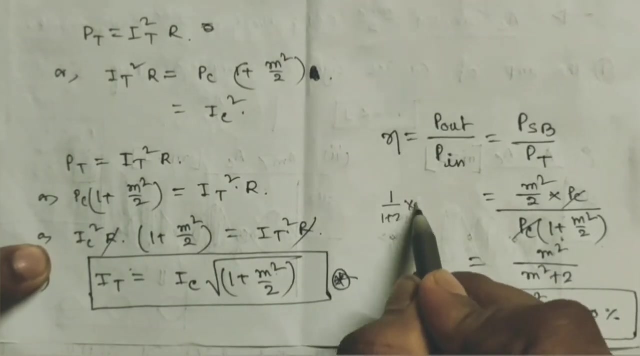 And hence more data is lost in amplitude modulation. Transmission requires more bandwidth and more power is consumed, And amplitude modulation has lesser frequency than frequency modulation. In this equation of efficiency, If we put m equals to 1, then eta will be 1 by 1 plus 2 into 100 percent. 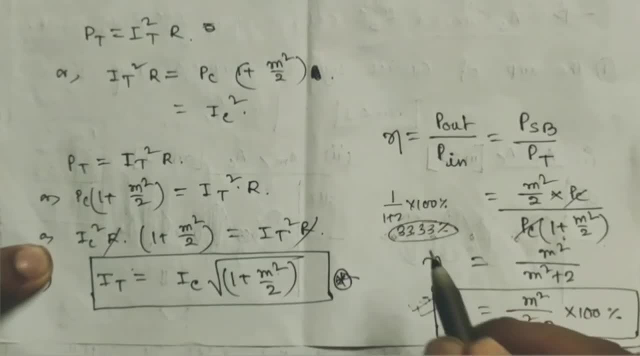 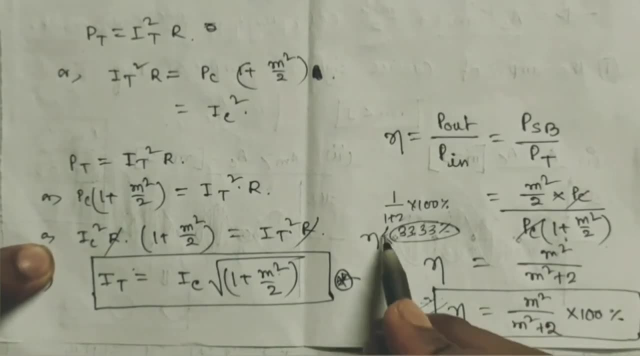 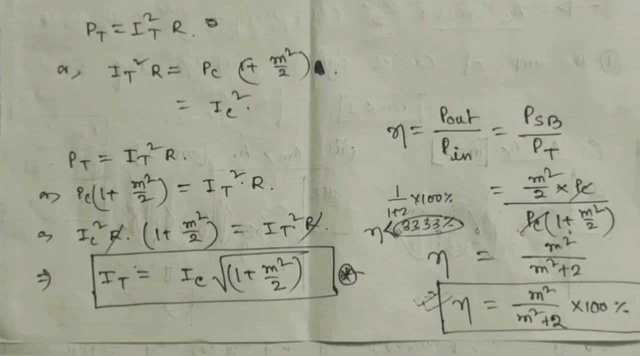 That is 33.33 percent. Now m value is always less than 1.. That is, eta value will be less than 33 percent, Which is very less and not desired, And hence, to get higher efficiency, we use angle modulation. In the next video we will learn about angle modulation. 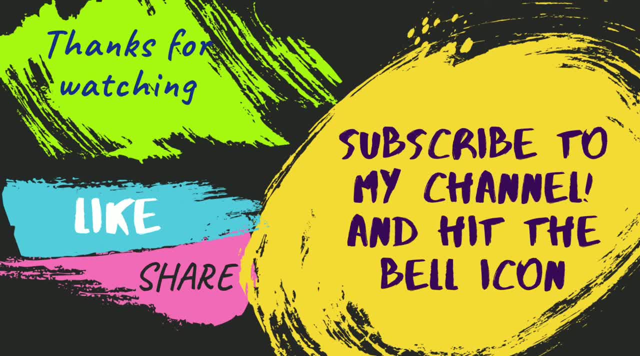 Thank you for watching. See you next time.